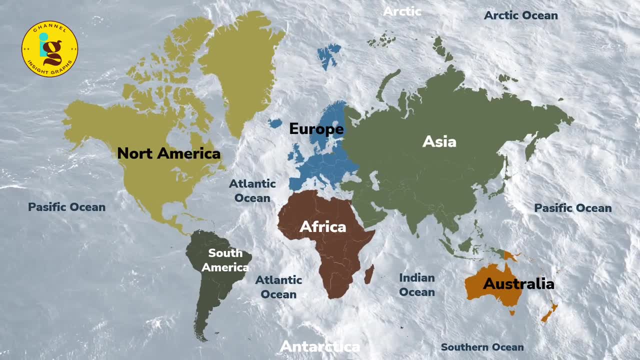 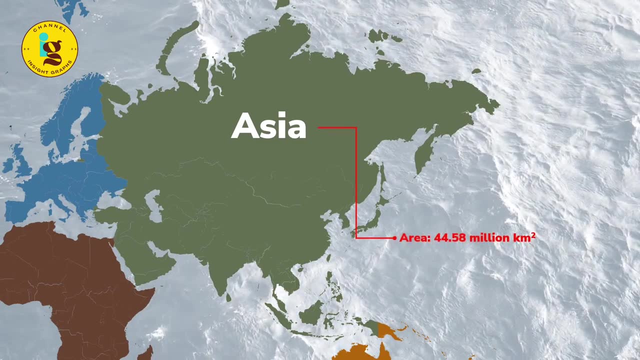 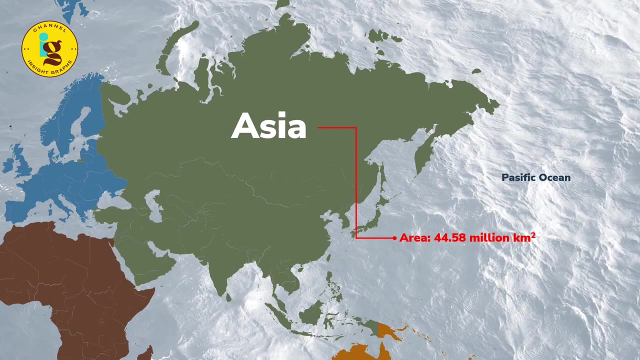 its size, shape and natural features. Asia is the largest continent on Earth, covering approximately 44.58 million square kilometers. Asia located primarily in the eastern hemisphere and is bordered by the Pacific Ocean to the east, the Arctic Ocean to the north and the 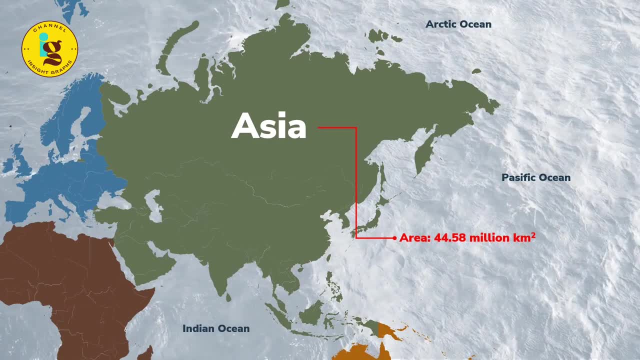 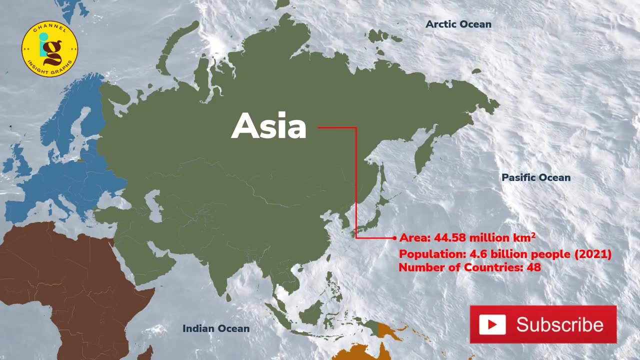 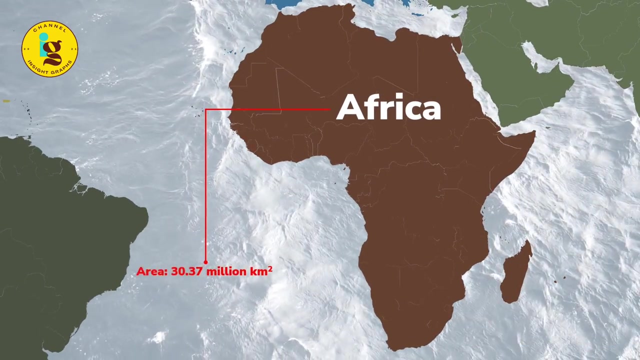 Indian Ocean to the south. It is also the most populous continent, with a population of over 4.6 billion people. Asia is home to 48 countries. Africa is the second largest continent on Earth, covering approximately 30.37 million square kilometers. It is located primarily in the eastern hemisphere and is bordered. 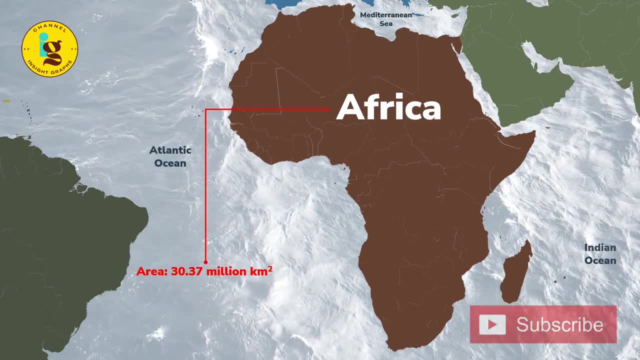 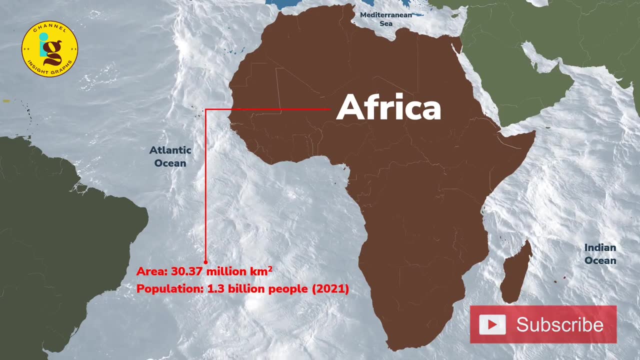 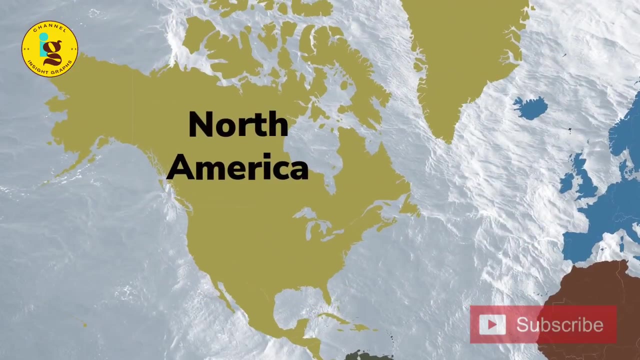 by the Mediterranean Sea to the north, the Atlantic Ocean to the west and the Indian Ocean to the east. It is the second most populous continent, with a population of over 1.3 billion people. Africa is home to 54 countries. 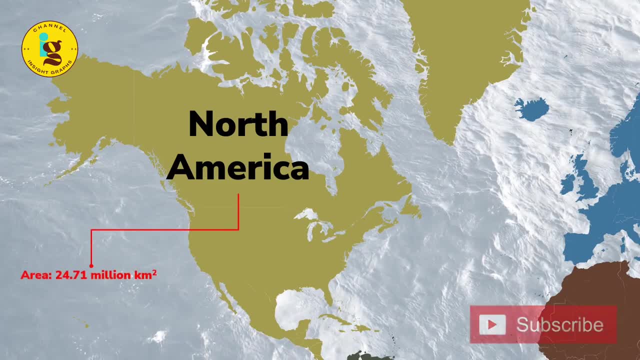 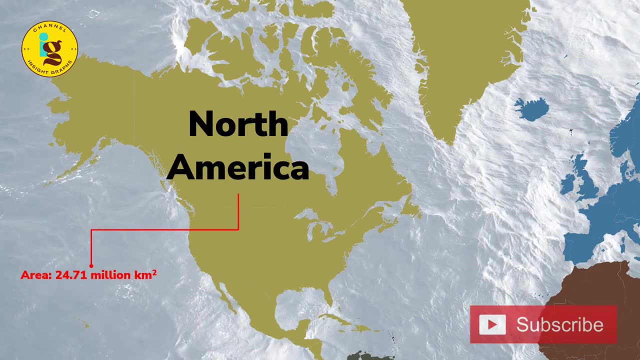 North America is the third largest continent on Earth, covering approximately 24.71 million square kilometers. It is located primarily in the northern hemisphere and is bordered by the Arctic Ocean to the south. Asia is the third largest continent on Earth, covering approximately 24.71 million square kilometers. It is located primarily in the northern hemisphere. 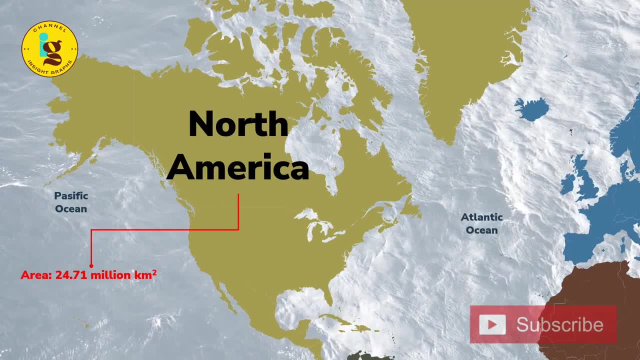 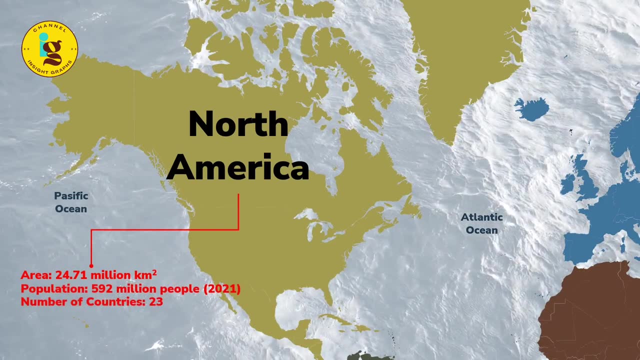 and is bordered by the Pacific Ocean to the west, the Atlantic Ocean to the south, the Pacific Ocean to the west and the Atlantic Ocean to the east. It has a population of over 592 million people and is home to 23 countries. 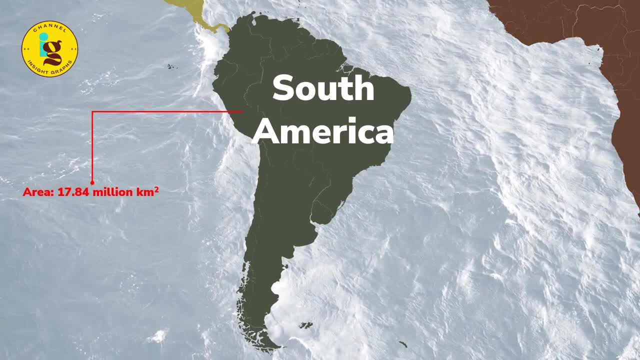 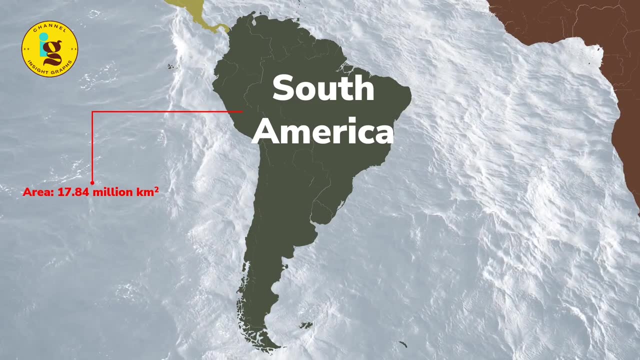 South America is the fourth largest continent on Earth, covering approximately 17.84 million square kilometers. It is located primarily in the southern hemisphere and is bordered by the Pacific Ocean to the west, the Atlantic Ocean to the east and the Southern Ocean to the south. 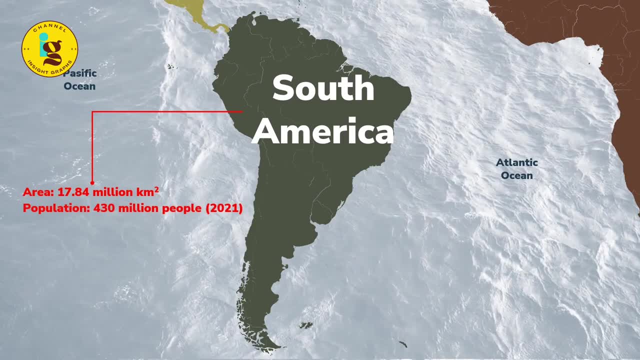 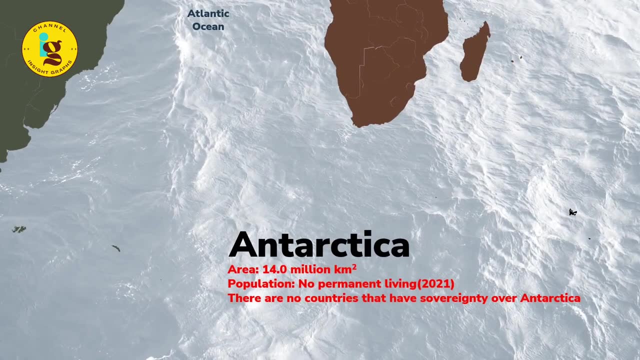 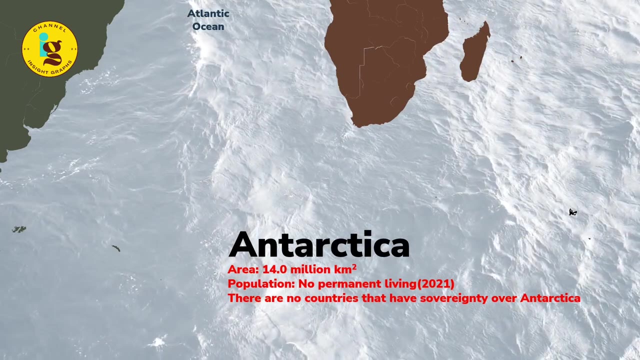 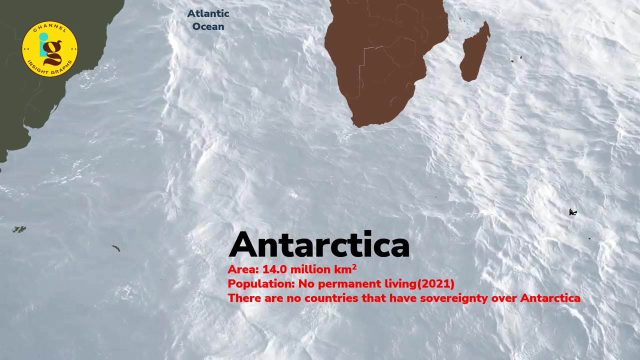 It has a population of over 430 million people and is home to 12 countries. Antarctica is the fifth largest continent on Earth, covering approximately 14.0 million square kilometers. It is located primarily in the southern hemisphere and is covered in ice and snow. It is the least populous continent, with no permanent residents, and